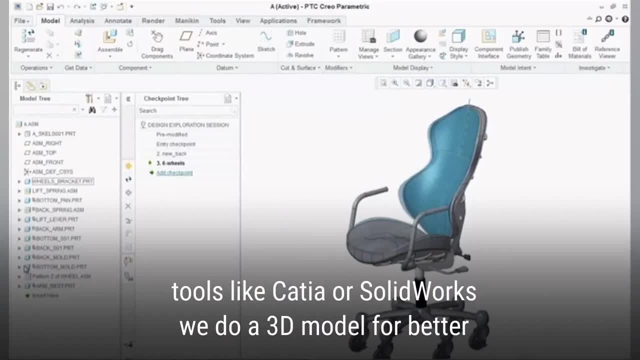 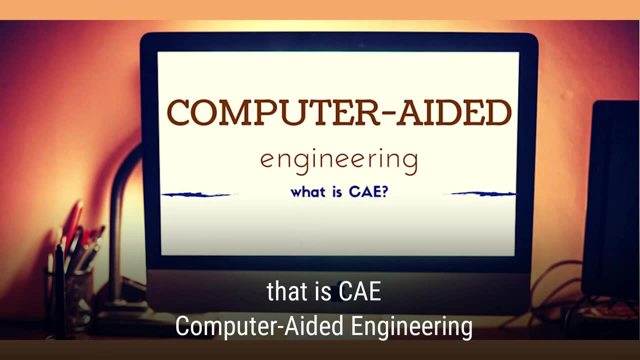 like CATIA or SOLIDWORKS, you do a 3D model for better visualization. Top 10 Softwares for Mechanical Engineers. Top 10 Softwares for Mechanical Engineers. Next phase is Design Optimization, that is, CAE- Computer Aided Engineering- wherein using 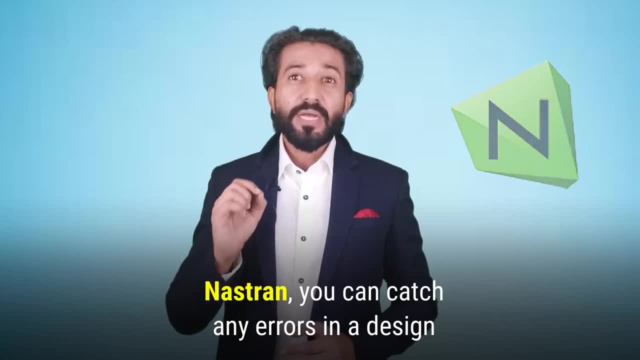 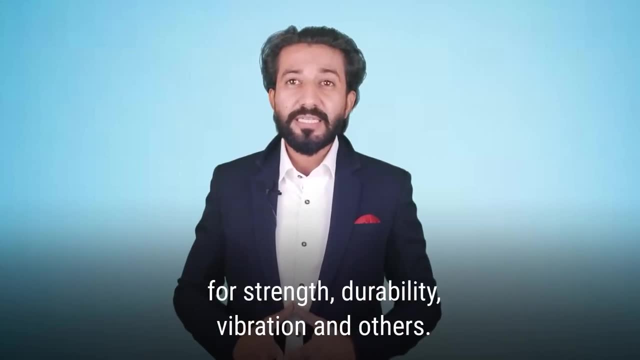 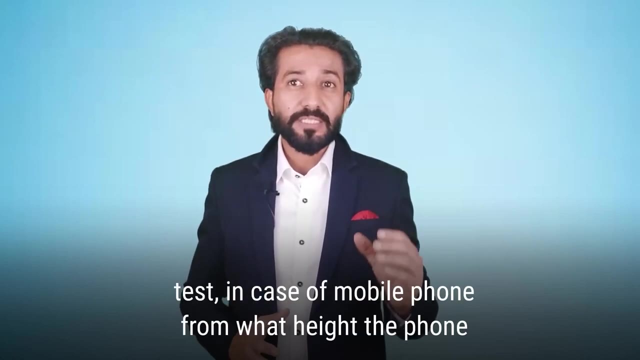 simulation softwares like ANSYS NASTRAN, you can catch any errors in your design before even building a physical prototype Example. you can check the model for strength, durability, vibration and others. You can also do various tests, like, say, for example, drop test in case. 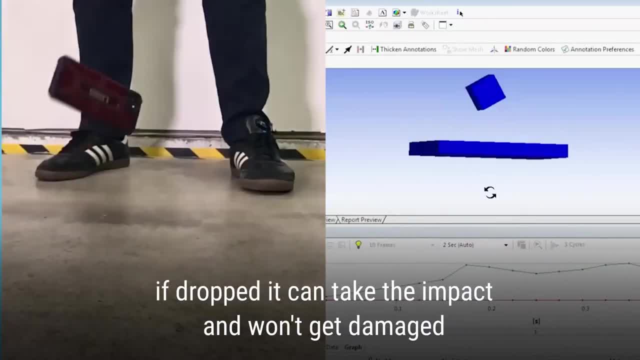 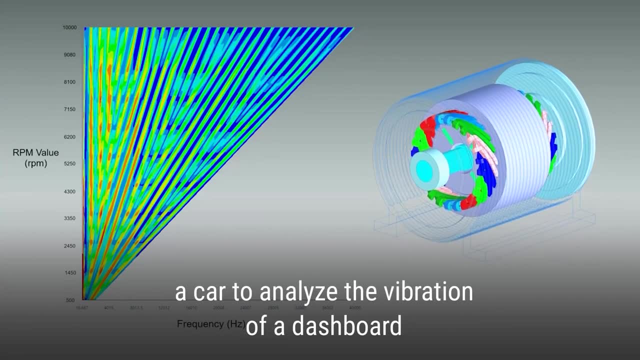 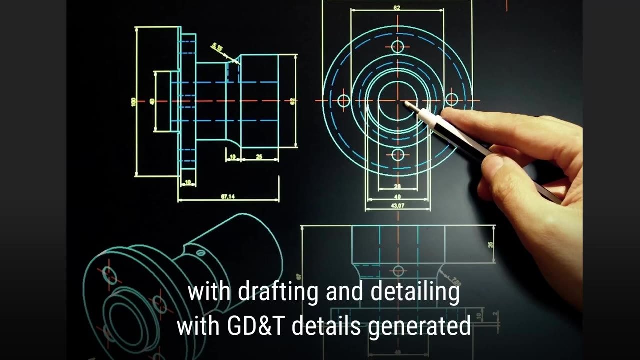 of mobile phone, from what height the phone, if dropped, it can take the impact and won't get damaged. or vibration analysis, in case of you driving a car to analyze the vibration of a dashboard, and if the result of the tests are okay, you proceed with drafting and detailing with GD&T details generated in 3D modeling software. 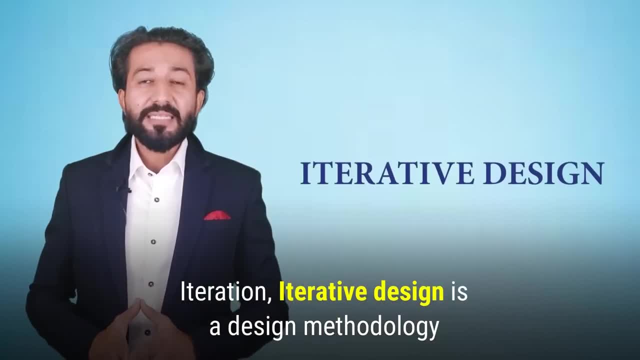 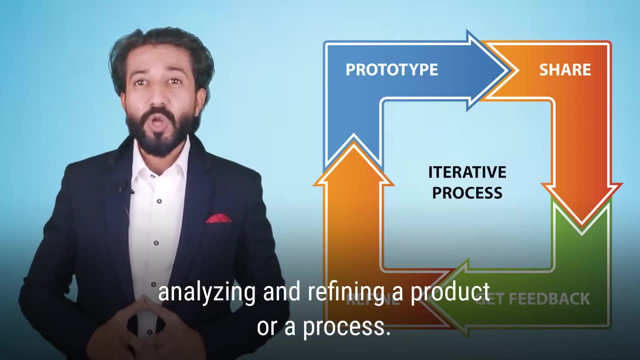 The third phase is Design Iteration. Iterative design is a design methodology based on cyclic process of prototyping, testing, analyzing and refining a product or a process. Once the design is iterative, it is a process of prototyping, testing, analyzing and refining a product or a process. 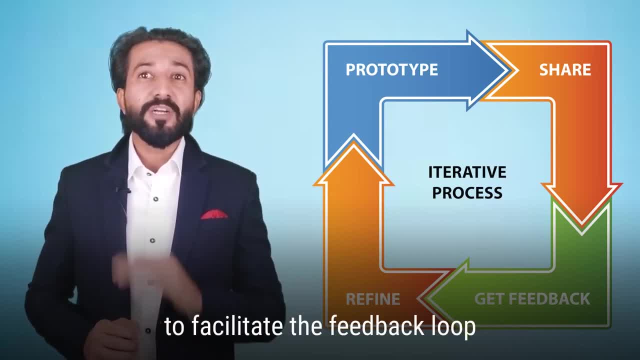 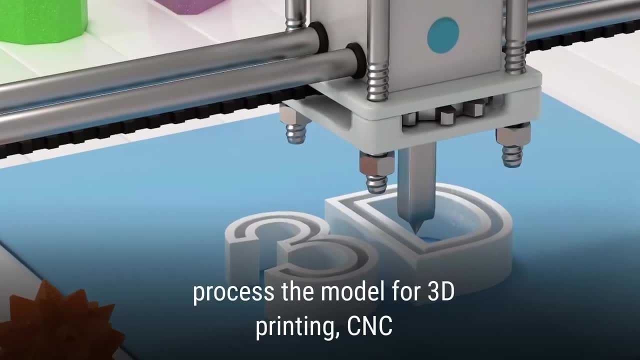 Once the design is iterative, the product could be rapidly prototyped to facilitate the feedback loop until the design finalization. By having a 3D model, you are able to quickly process the model for 3D printing, CNC machining and so on. Let's look at an example. This is a modeling of a fork. 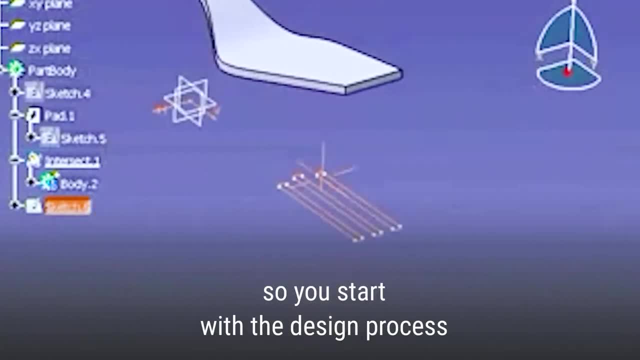 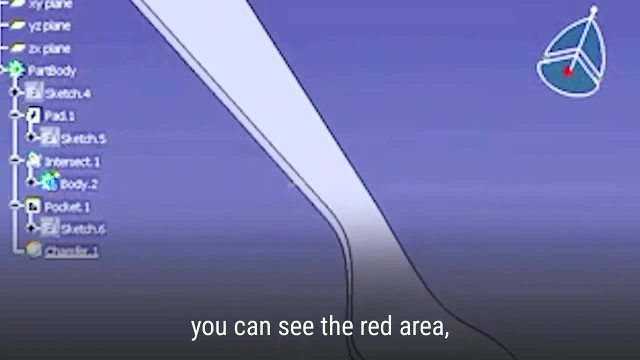 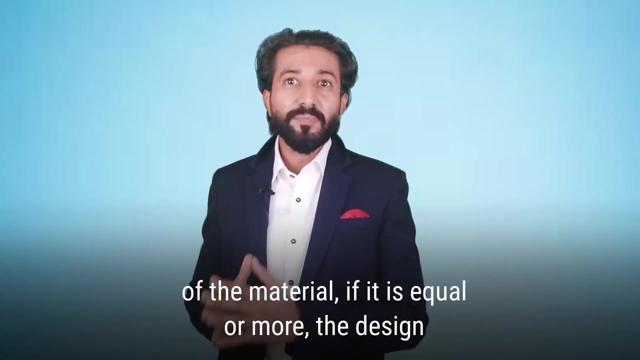 spoon. So you are starting with the design process. You want to model it. We are using for this CADIA software and once it is modeled you can see the red area. This is the area where maximum stress occurs and we compare it with yield strength of the material If it is equal. 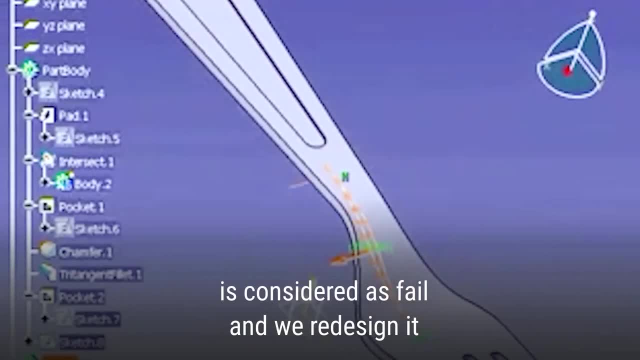 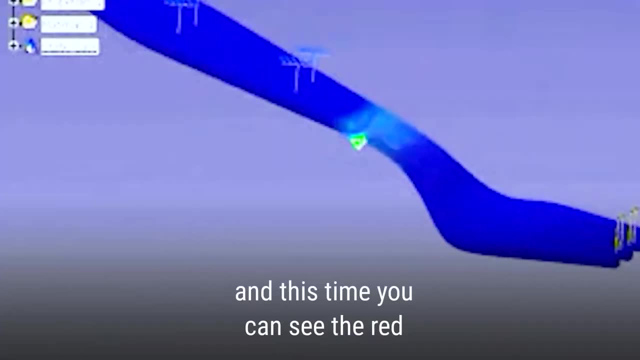 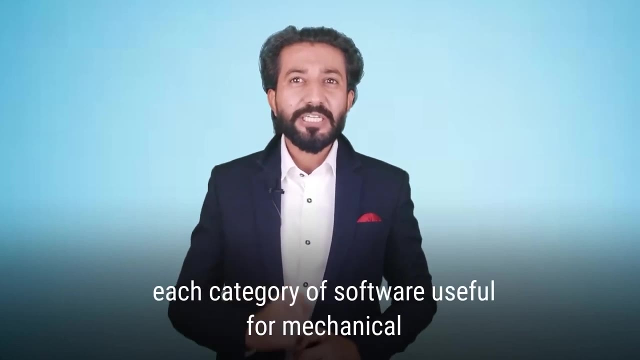 or more, the design is considered as fail and we redesign it again and provide more strength at the bridge, and we run the analysis again and this time you can see the red part is not visible or it is reduced when we apply load to it. Now let's explore each category of software. 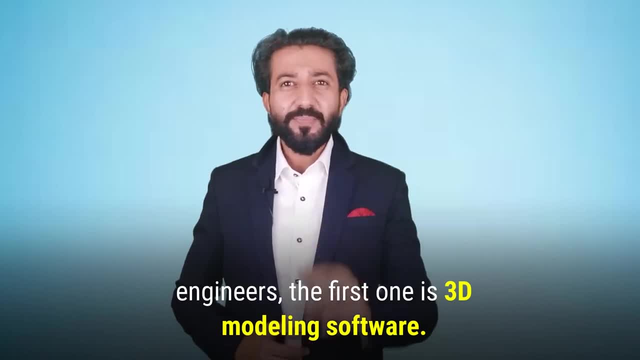 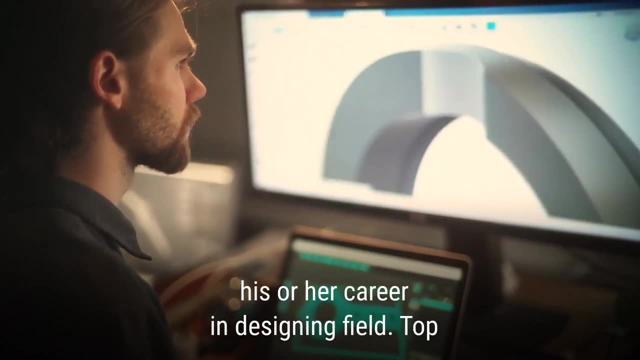 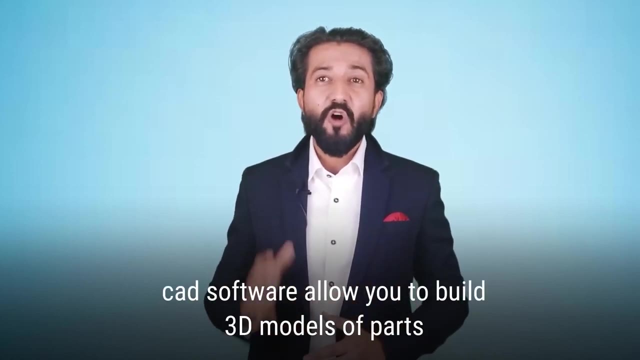 useful for mechanical engineers. The first one is 3D modeling softwares. CAD software is essential for one who wants to make his or her career in designing field. Top five benefits of learning CAD software are: CAD software allows you to build 3D models of parts and assemblies, For instance. 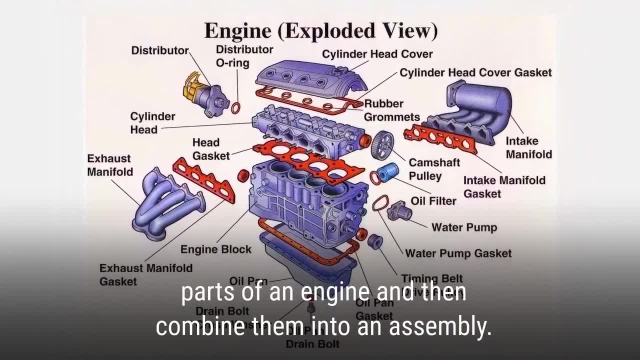 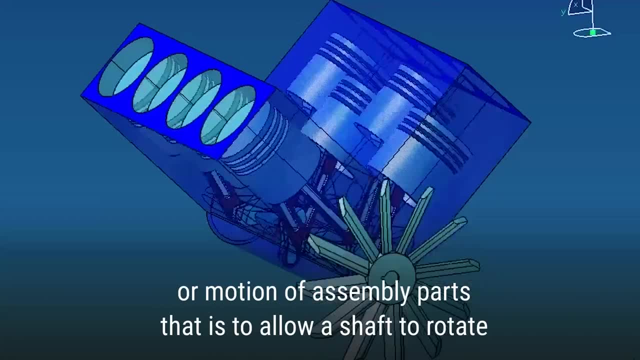 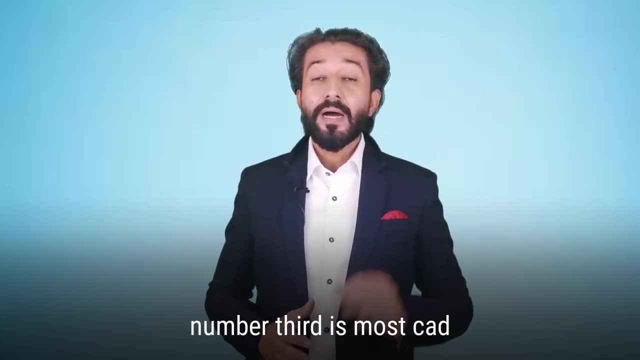 you could model all of the individual parts of an engine and then combine them into an assembly. Many CAD packages allow you to do simulation or motion of assembly parts. that is, to allow a shaft to rotate and to check for interferences between the parts. Most CAD packages have a drafting component. 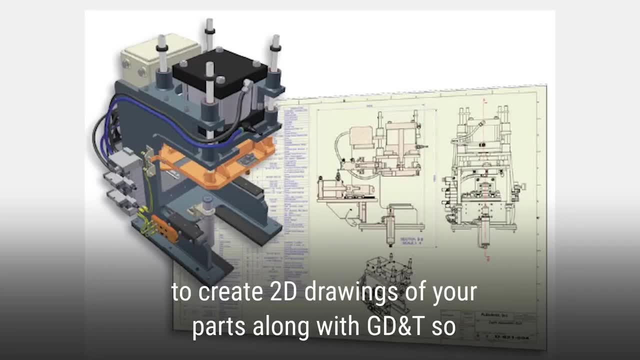 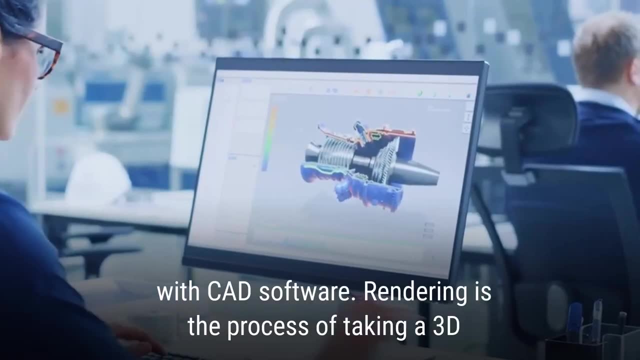 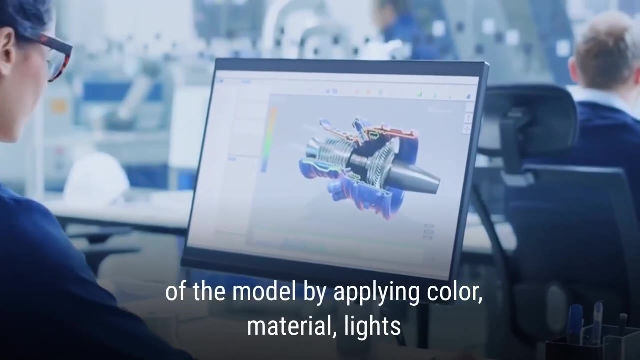 that allows you to create 2D drawings of your parts along with GD&T so that they can be manufactured. You can also do rendering with CAD software. Rendering is the process of taking a 3D model and generating a photorealistic representation of the model by applying color material. 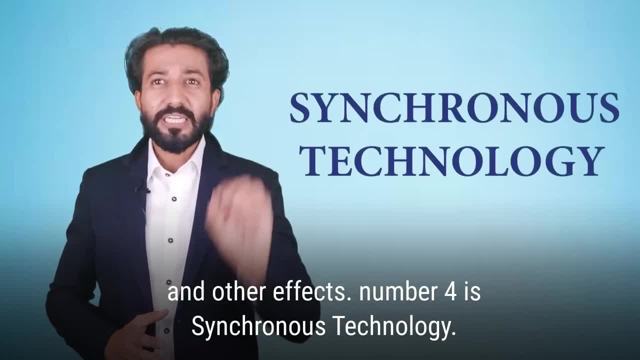 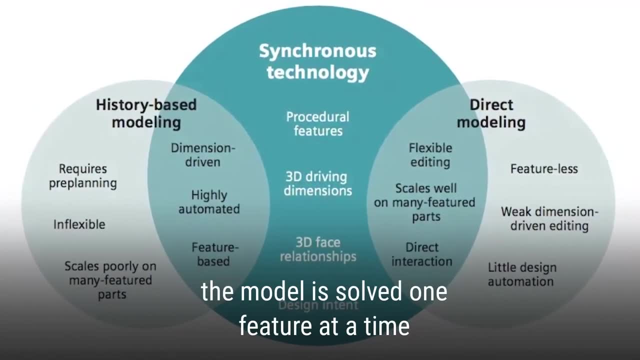 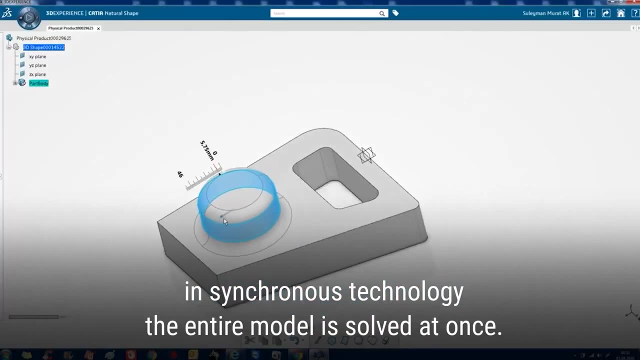 lights and other effects. Number fifth is synchronous technology. It's the latest thing in 3D modeling. In a history-based CAD tool, the model is solved one feature at a time and each successful feature is added to the body. In synchronous technology, the entire model is solved at once. 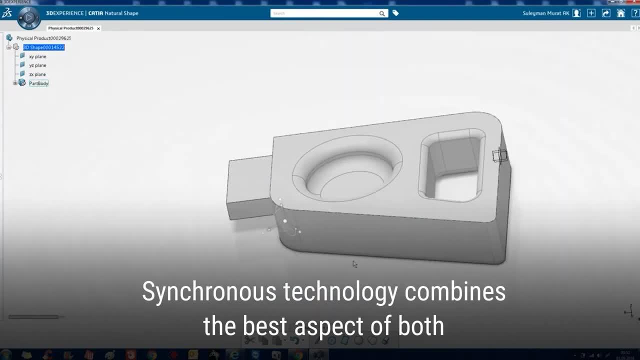 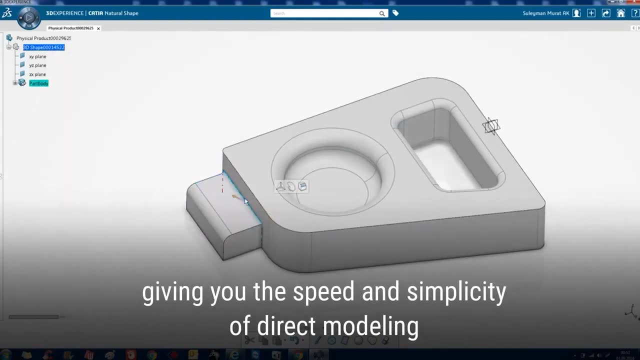 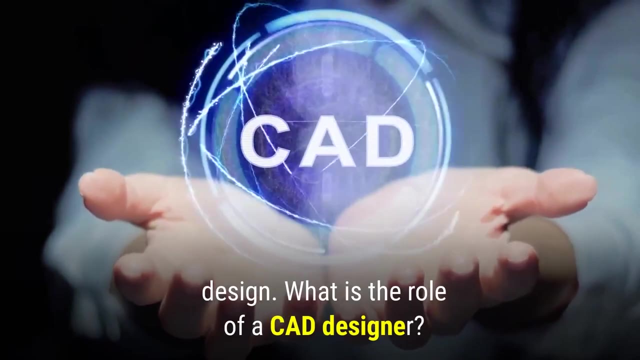 Synchronous technology combines the best aspect of both history-based models and direct modeling approaches, giving you the speed and simplicity of direct modeling while still having the best control and intelligence of history-based design. What is the role of a CAD designer? The first one is data collection, then 2D and 3D modeling and detailing. 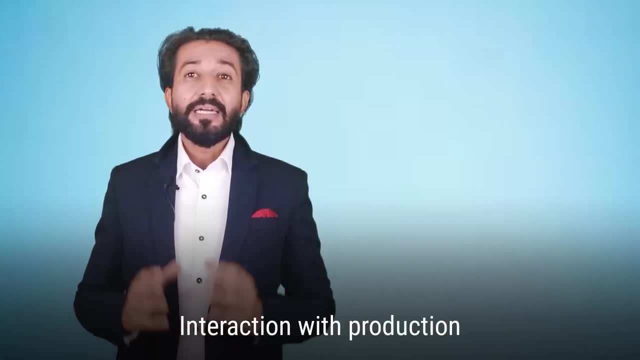 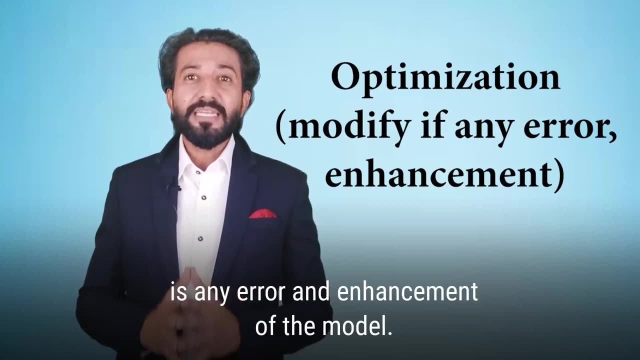 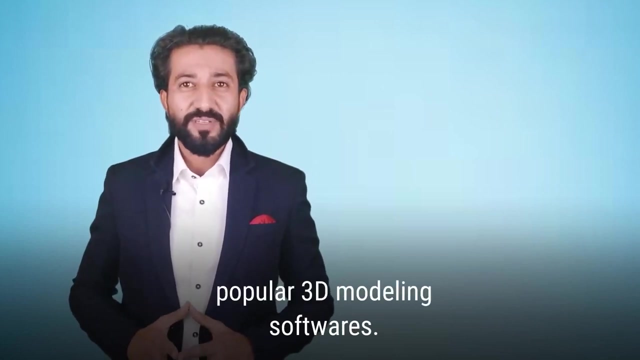 that is, process, dimensioning and tolerances, interaction with production and quality department and the vendor. and optimization, that is, modify if there is any error and enhancement of the model. Now let's look at what are the most popular 3D modeling softwares. 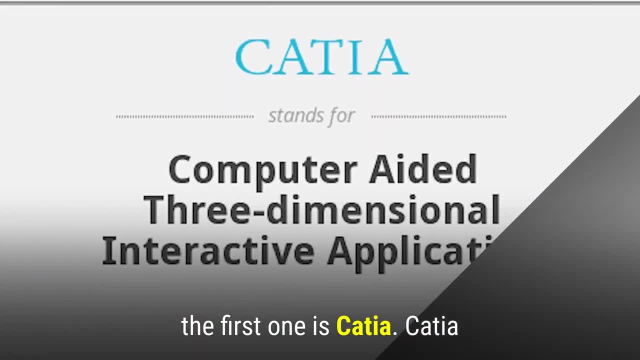 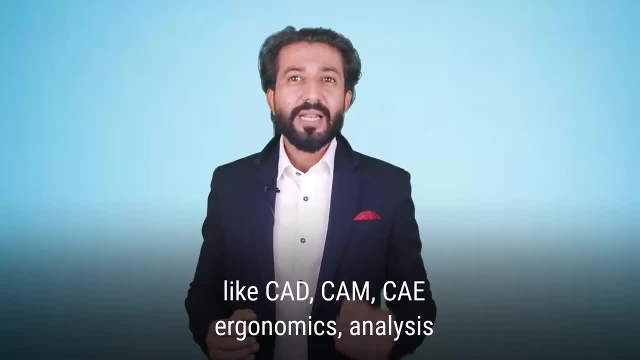 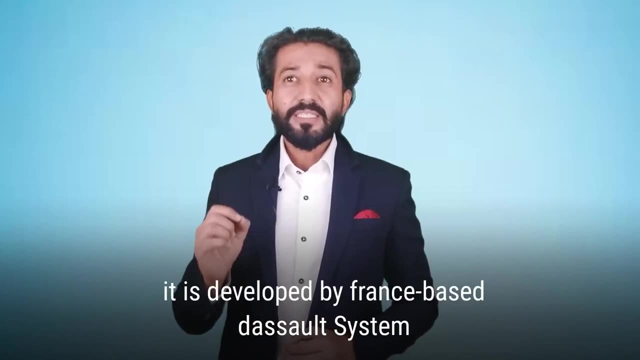 The first one is CATIA. CATIA is a product lifecycle management, that is, a PLM software, which have all required tools like CAD, CAM, CAE, ergonomics analysis, CFD, etc. It is developed by France-based Dassault Systèmes, mostly used for aerospace composite design. 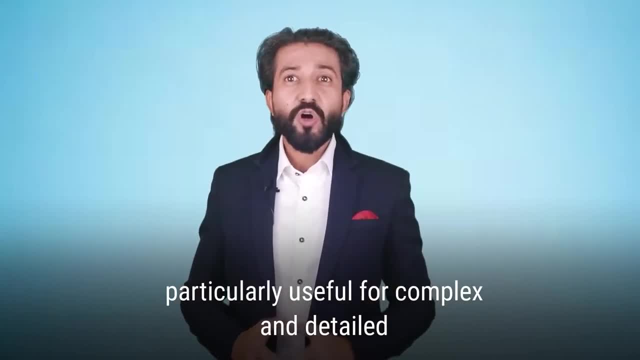 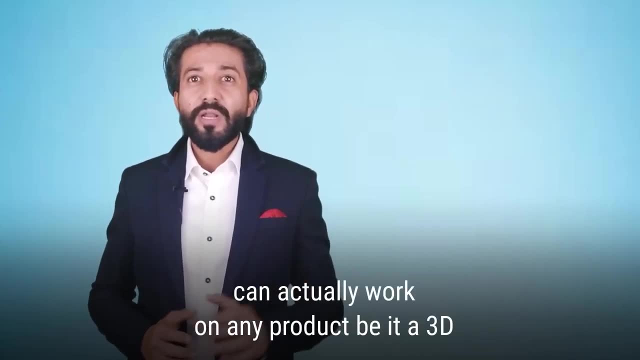 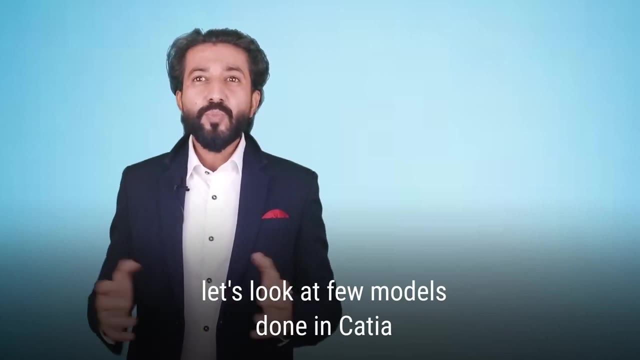 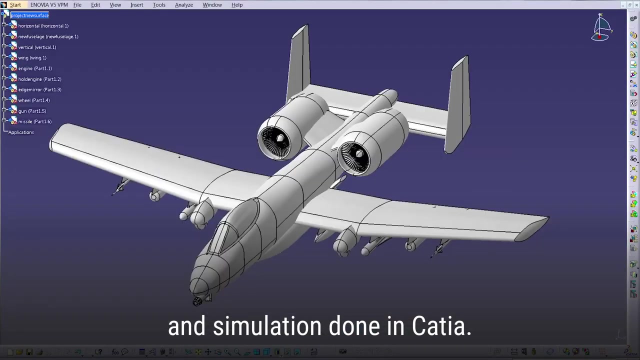 and automotive projects, Particularly useful for complex and detailed design of a surface, greatly fazendo creasing and Hyun-Yum TA and sheet extra metal, So for doingเห recib And CATIA, is used to design and process interesting components such as every kind of wood metal and before it can work. 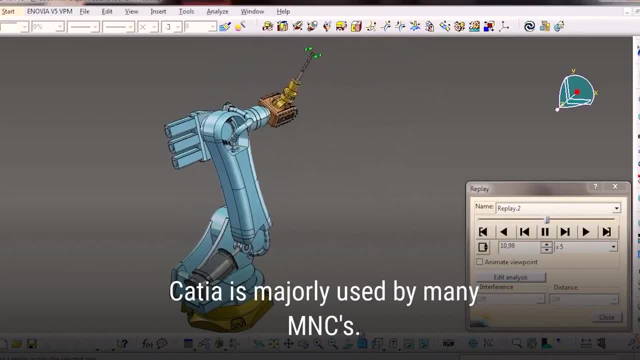 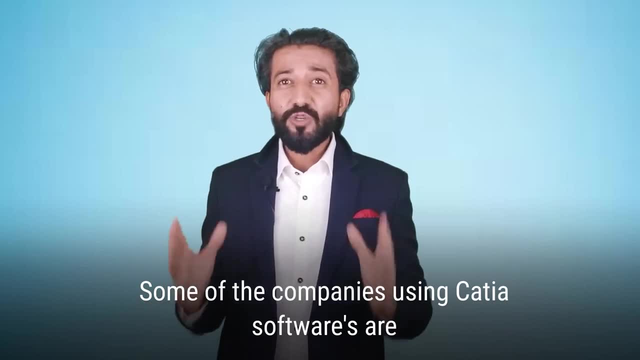 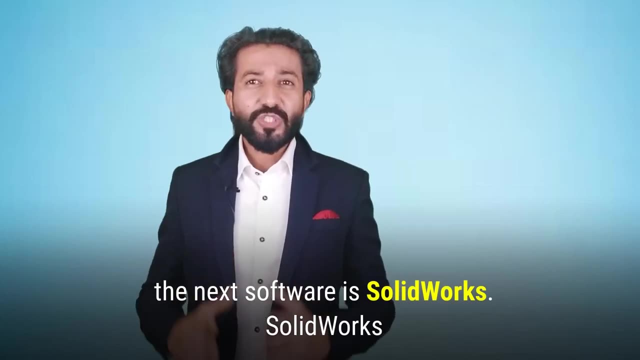 In CATIA you can actually work on any product, be it 3D CAD models, used by many MNCs. Some of the companies using CATIA softwares are: The next software is SOLIDWORKS. SOLIDWORKS will perfectly fit engineering students looking. 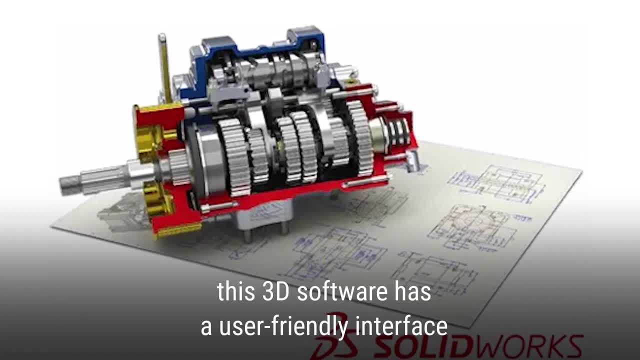 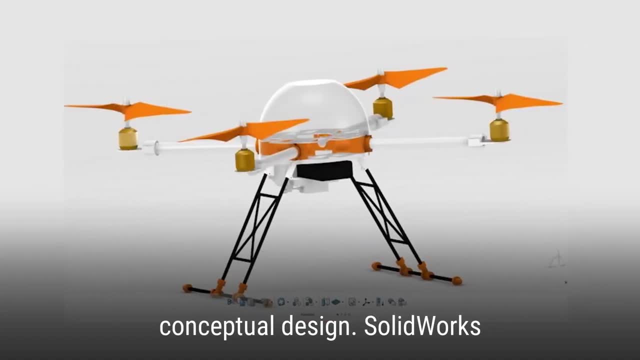 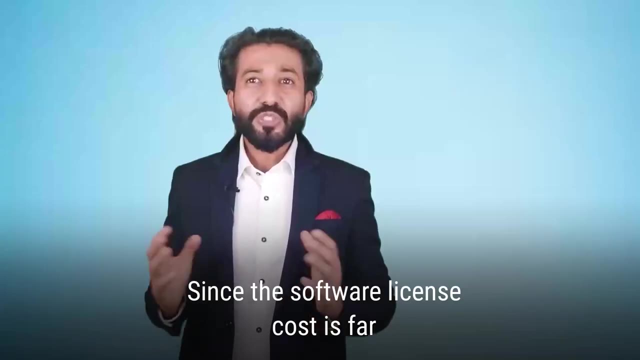 for a great tool to make mechanical drawings. This 3D software has a user-friendly interface and can be used to create machinery parts or conceptual design. SOLIDWORKS could enable you to work on specific parts, such as a car engine, Since the software license cost is. 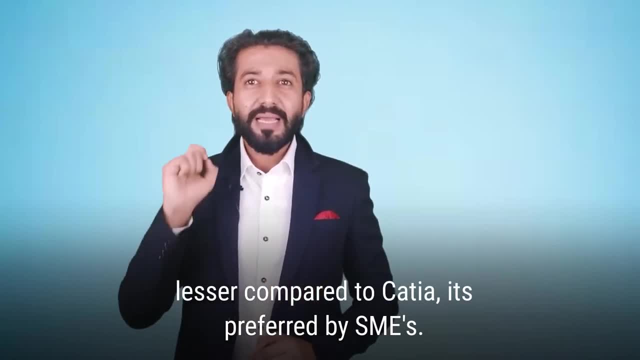 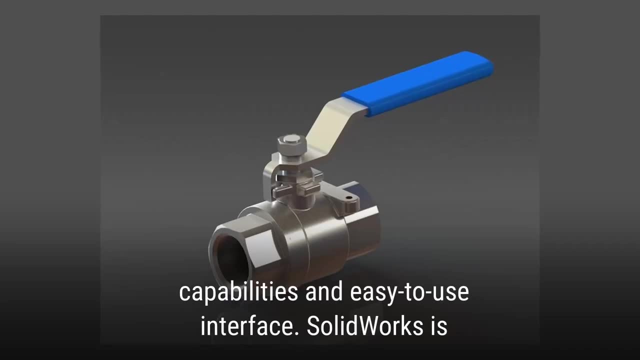 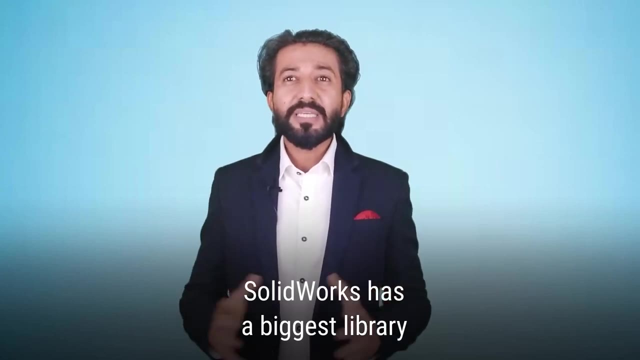 far lesser compared to CATIA. it is preferred by SMEs. The strength of this software is its rendering capabilities and easy-to-use interface. SOLIDWORKS is primarily used for small-scale and simpler design projects. SOLIDWORKS has the biggest library of fasteners, which are grouped according to the standards and types. 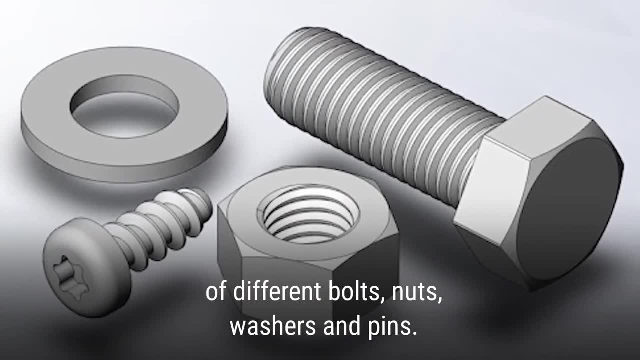 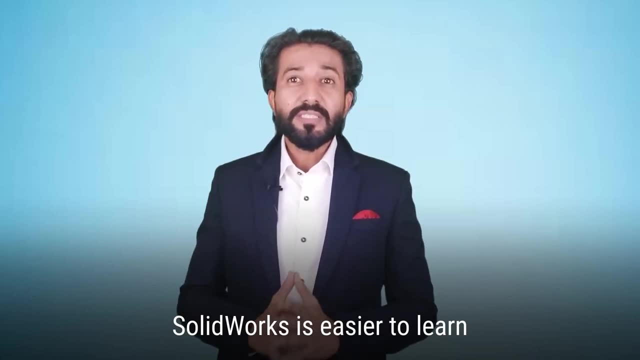 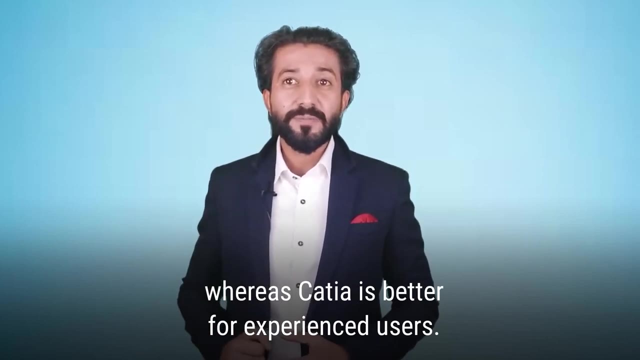 It range of different bolts, nuts, washers and pins. The main differences between SOLIDWORKS and CATIA are: SOLIDWORKS is easier to learn and more suitable for beginners, whereas CATIA is better for experienced users. SOLIDWORKS is designed particularly for 3D solid object. 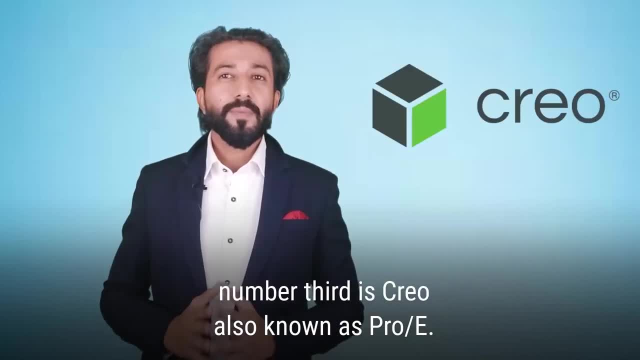 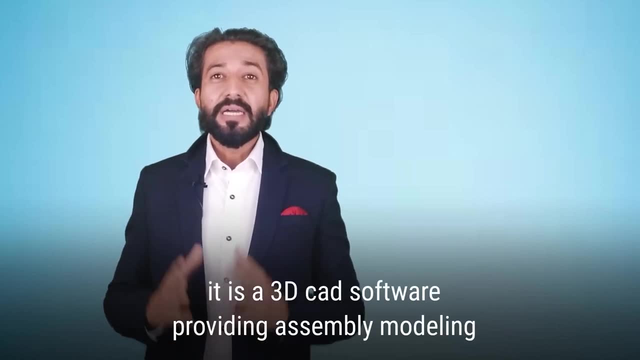 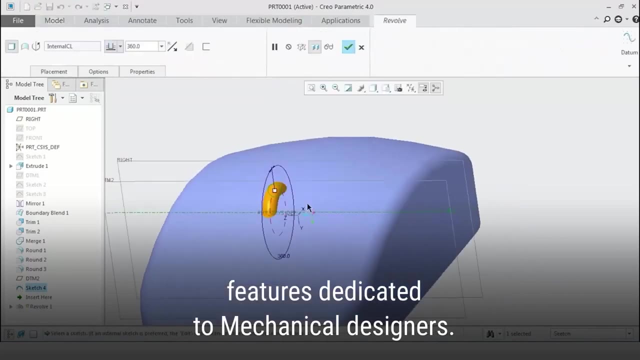 modeling, whereas CATIA is an all-rounder. 3. CREO, Also known as PRO-E, developed by Parametric Technology Corporation, It is a 3D CAD software providing assembly modeling, nerve surface modeling. It has also great features dedicated to mechanical designers. 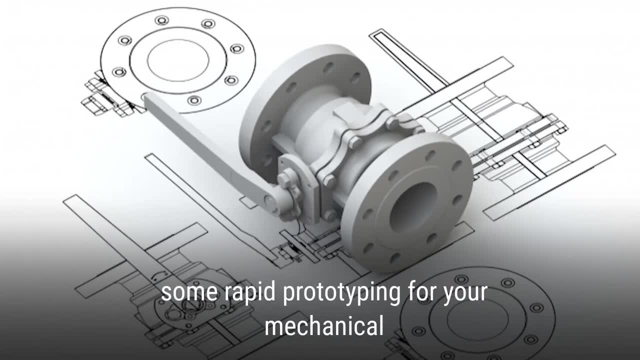 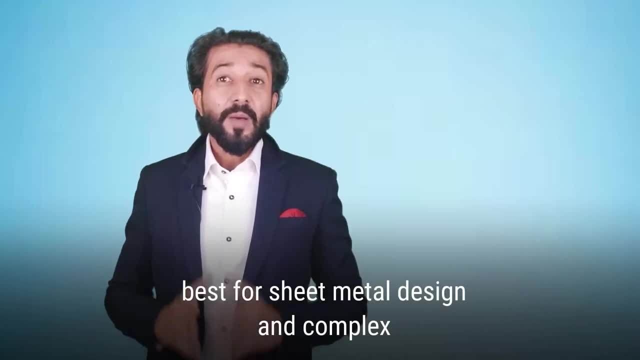 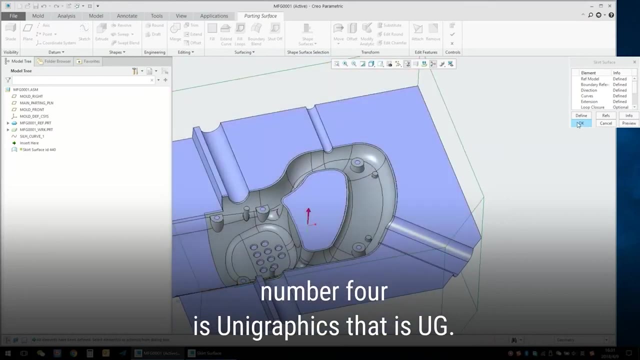 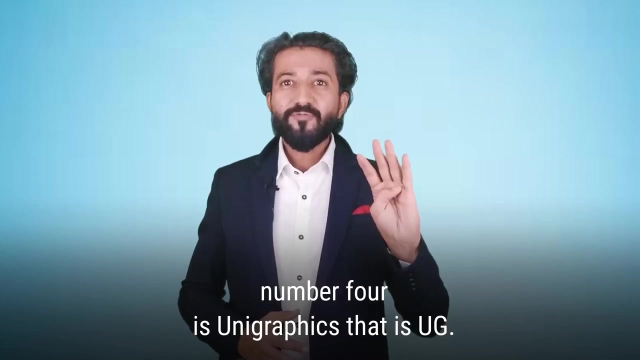 This is a good and complete software solution to do some rapid prototyping for your mechanical projects and parts and also to produce your end-use products, Best for sheet metal design and components. 4. UGNX. UGNX is developed by Siemens PLM Software. 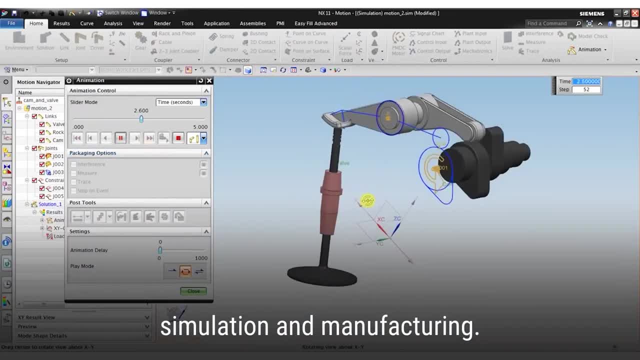 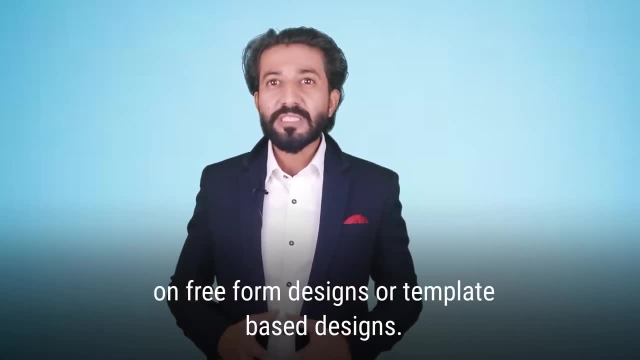 allowing you to work on conception, simulation and manufacturing. This software solution will provide you with all the necessary tools to work on free-form designs or 3D modeling. This software tool also allows you to work on sheet metal parts, For example. you can 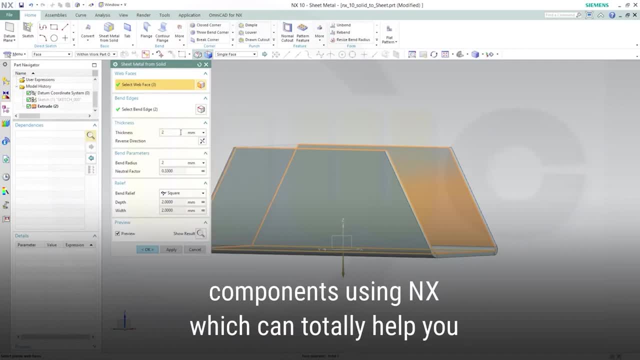 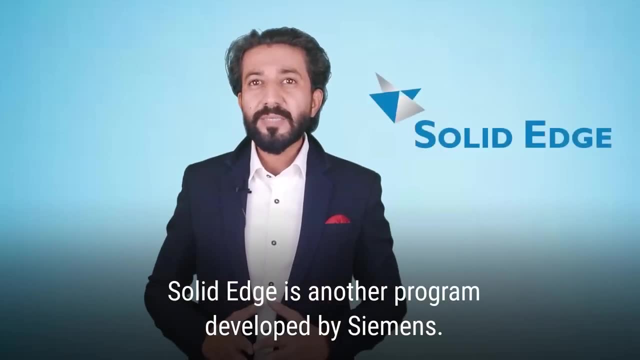 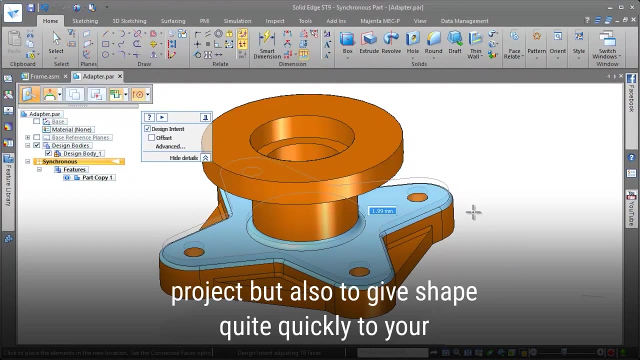 quickly convert a solid model to sheet metal components using UGNX, which can totally help you with your technical projects. 5. SOLIDAGE: SOLIDAGE is another program developed by Siemens. It is a perfect 3D software for engineers for complex projects, but also to give shape quite quickly to your ideas. It. 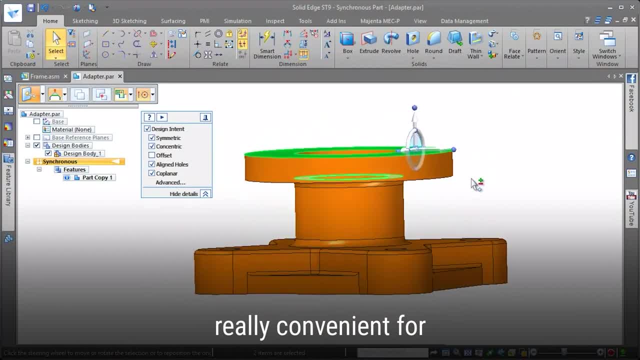 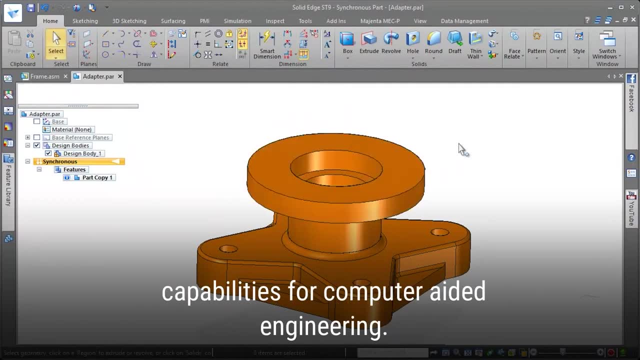 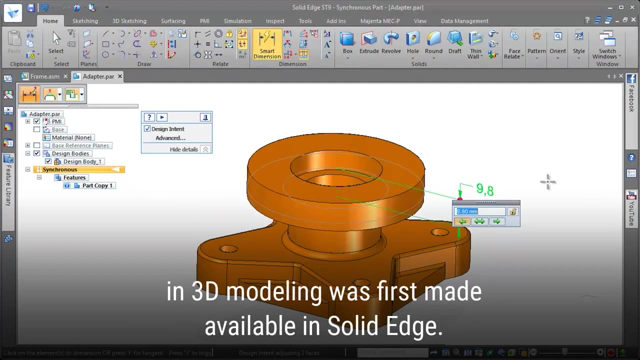 has great tools to help you with your technical projects. This software tool also allows you to work on 3D orthographic view functionality- really convenient for mechanical designers. It also has powerful engineering simulation capabilities for computer-aided engineering. Synchronous technology- the revolutionary technology in 3D modeling, was first made. 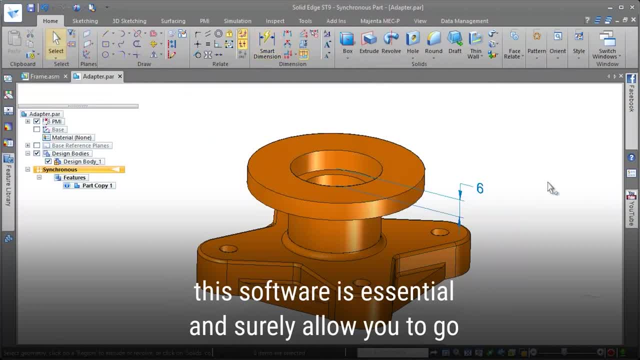 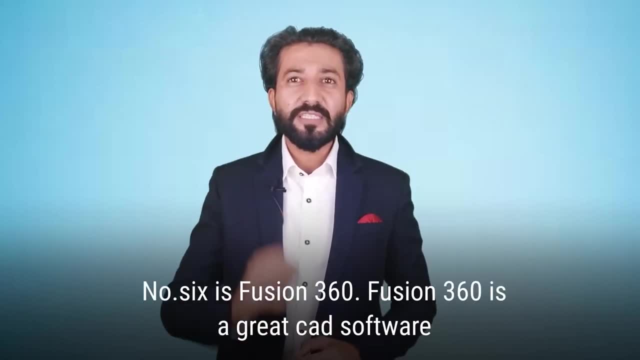 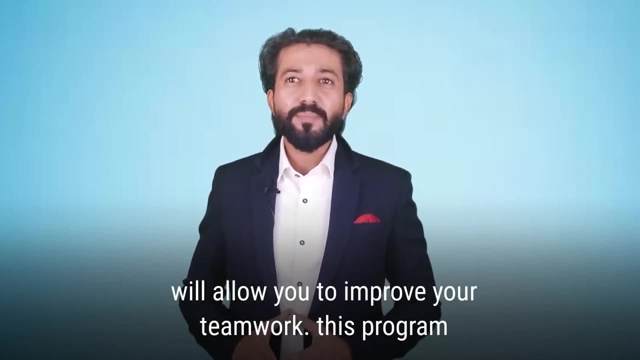 available in SOLIDAGE. This software is essential and will surely allow you to go further with all of your technical 3D projects. 6. FUSION 360: FUSION 360 is a great CAD software software tool developed by Autodesk. This is a cloud-based program that will allow you to improve your 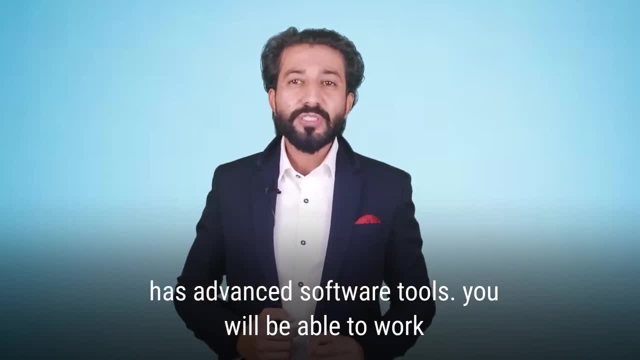 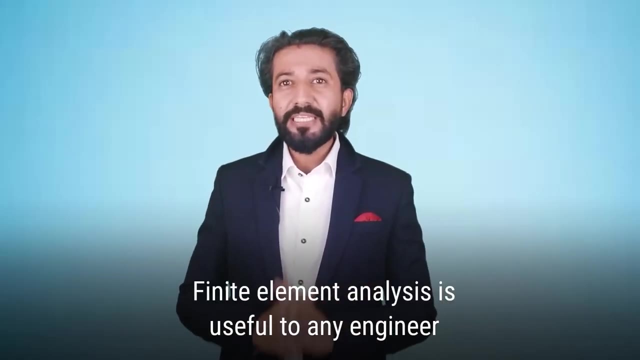 teamwork. This program has advanced software tools. You will be able to work on solid modeling, mesh modeling and parametric modeling 7.. The next category of software is FINITE ELEMENT ANALYSIS, that is, FES software. FINITE ELEMENT ANALYSIS is useful to any engineer that needs to perform structural analysis. This software allows you to analyze stresses and deflections in a 3D model. This software is also used in 3D modeling. 8. FUSION 360. FUSION 360 is a great CAD software tool that will allow you to go further with 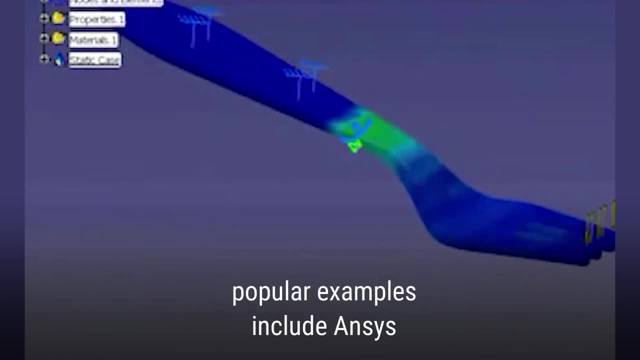 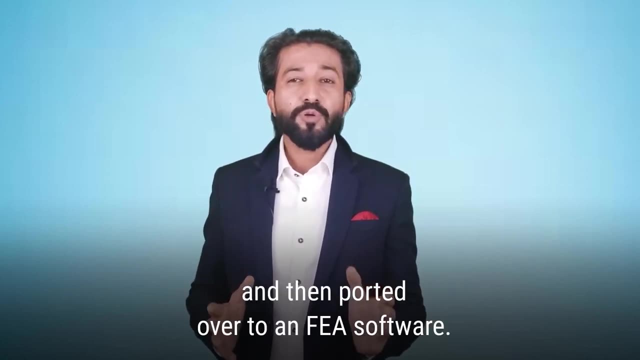 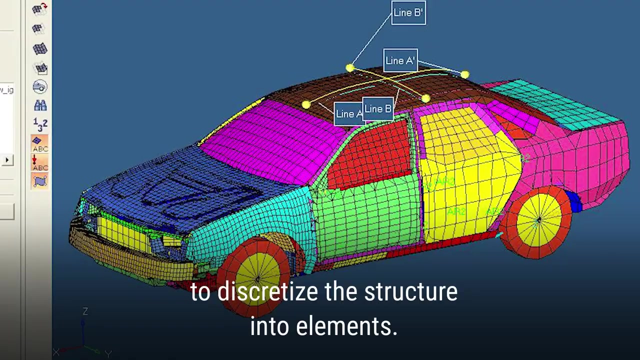 complex structures. Popular examples include ANSYS and NESTRAN. Typically, a structure will be modeled in a 3D CAD program and then ported over to an FES software. Once the geometry is built, a mesh is created to discretize the structure into elements. This can be done. 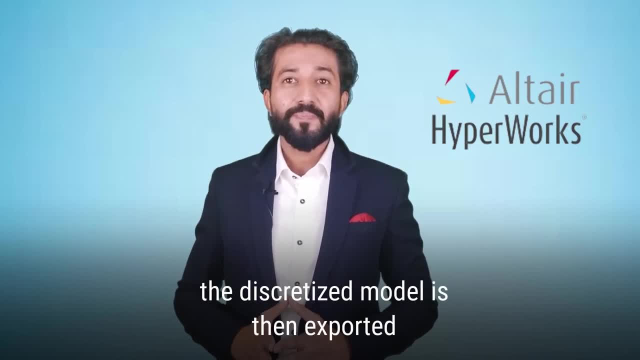 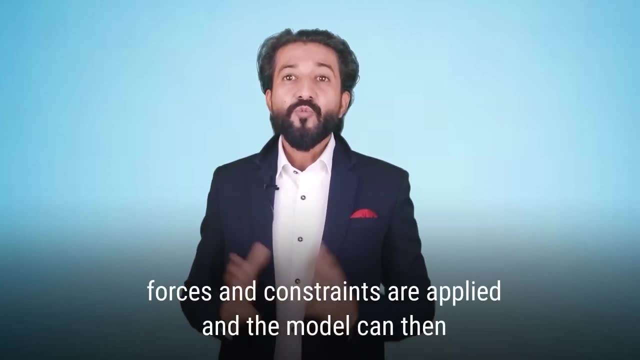 using exclusive meshing software called HYPERMESH 9.. The discretized model is then exported to an analysis package like ANSYS 10.. The discretized model is then exported to an analysis package like ANSYS 11. The software helps machines the greater impact of mass distribution to the mirror. 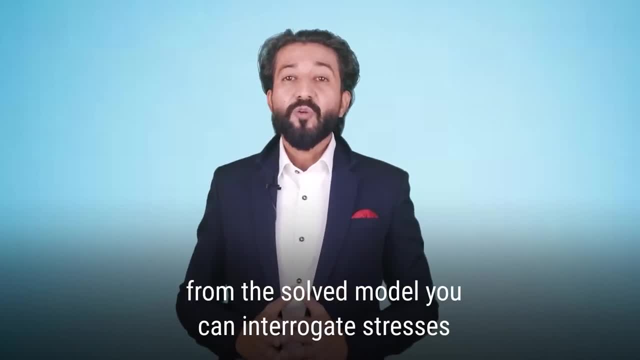 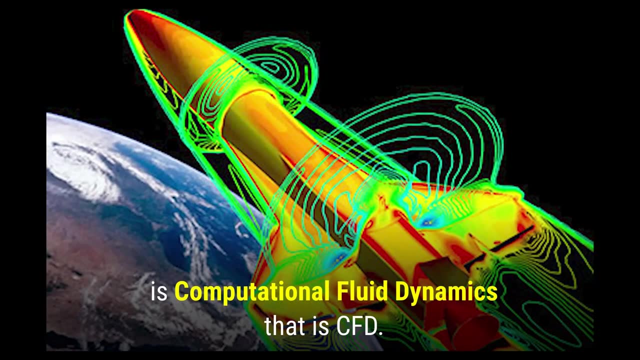 and becomes more precise and much easier to solve. 12. FOS is the process of creatingaziose parts 13 to 14ibly. 14 candidates are trained to be executed at least once a year. 14 day planning of working stages in a site. 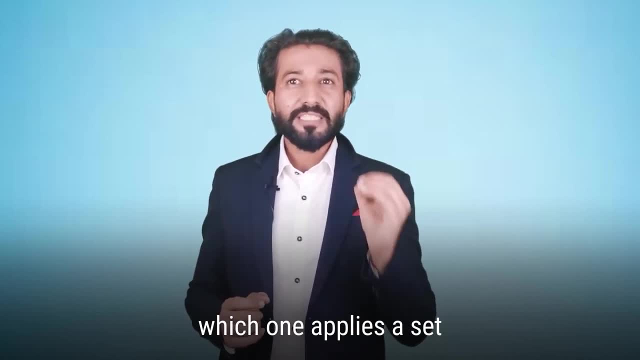 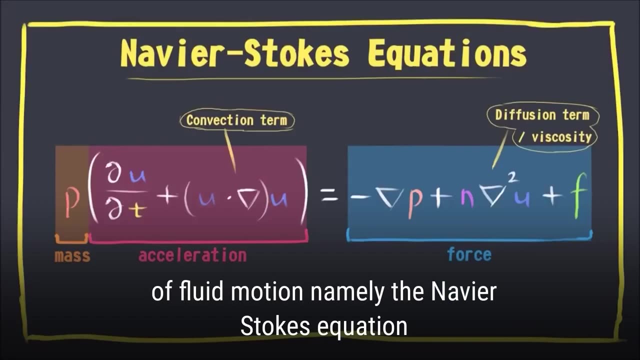 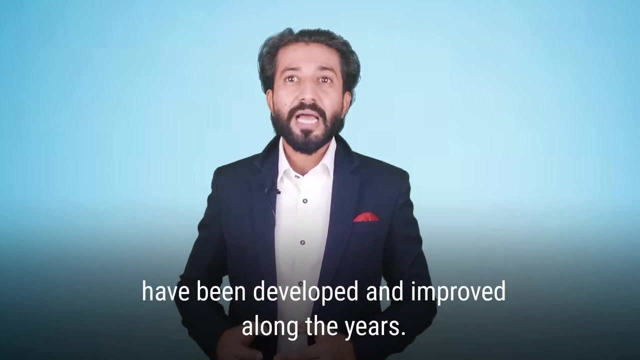 where a model on 6x1 scale universe is implemented. 14- NNC is the Data Evaluation restructure. 14. NNC is the思ema measuring step for all the compositions being applied. By applying such techniques, aided by computer programs, many CFD codes or solvers have been 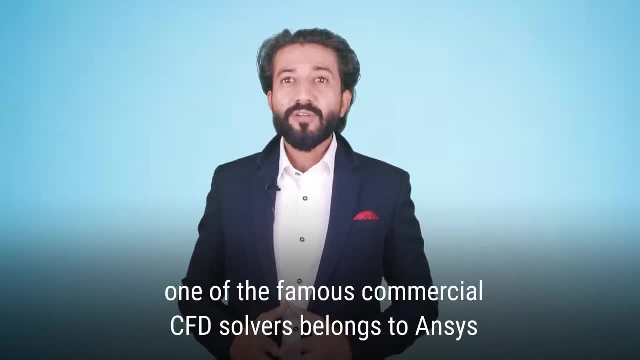 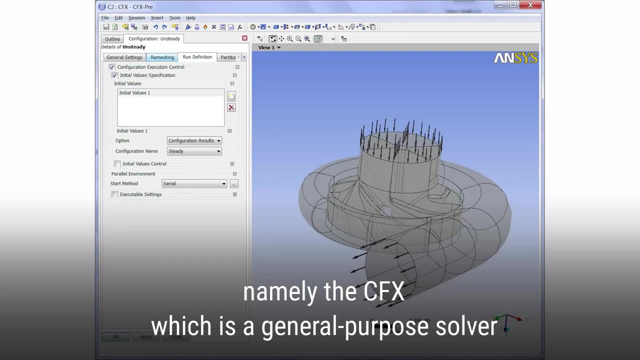 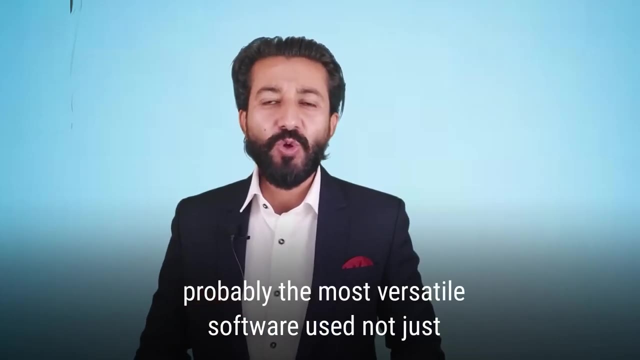 developed and improved along the years. One of the famous commercial CFD solvers belongs to ANSYS, namely the CFX, which is a general purpose solver for fluid flows. 9. Microsoft Excel: Excel is probably the most versatile software, used not just by mechanical engineers but by nearly every office worker. 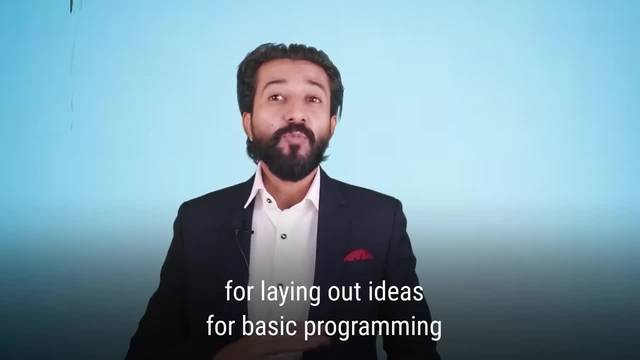 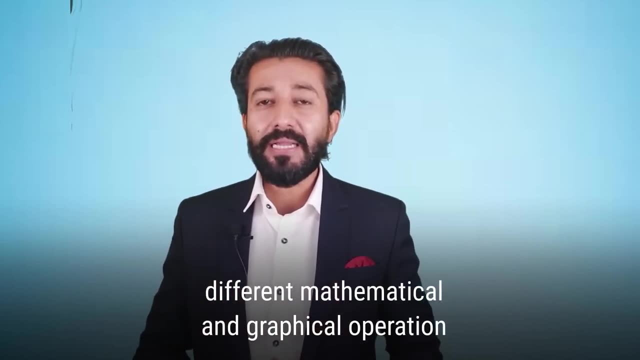 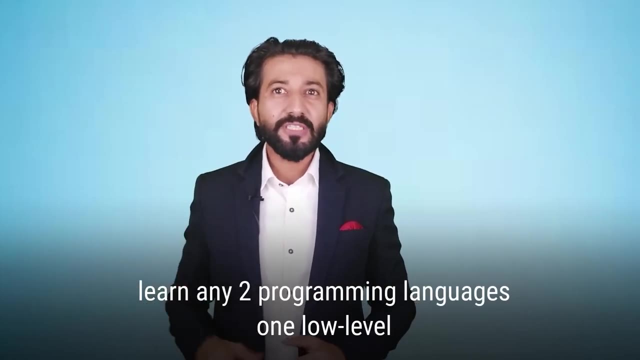 Excel is used for quick calculations, for tabulating data, for laying out ideas for basic programming. The possibilities are endless. You can perform different mathematical and graphical operations regarding engineering topics. 10. Coding Software: Learn any two programming languages, one low. 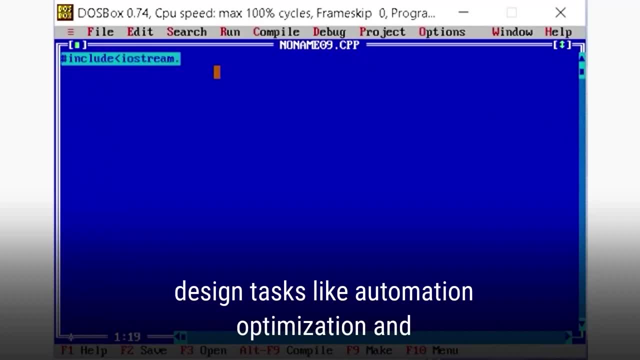 level and another high level, which will help you in many design tasks like automation, optimization and so on, Preferably C++ and MATLAB. Low-level languages like C, C+, Python and C++ Python will be useful in writing scripts for automation and to use customized functions. 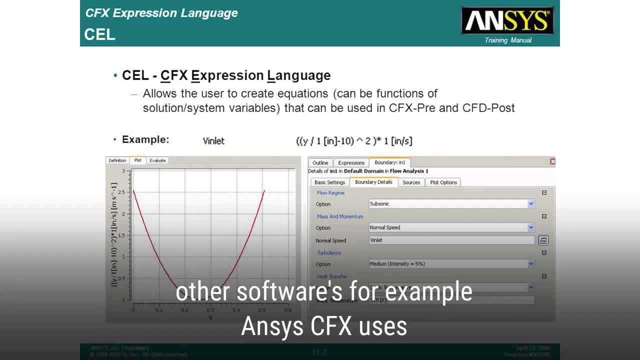 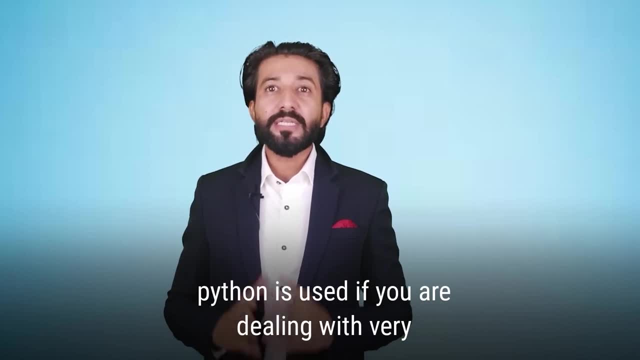 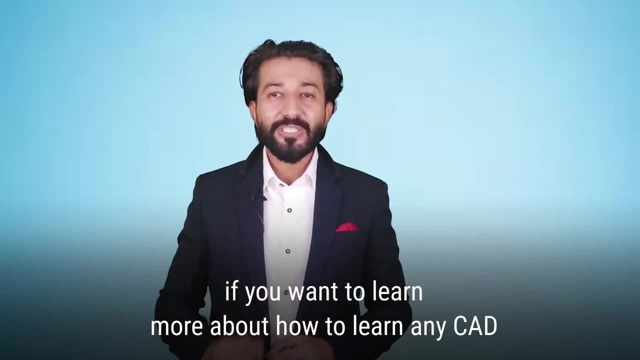 in other softwares. For example, ANSYS CFX uses Fortran as scripting language and ANSYS Fluent uses C+. Python is used if you are dealing with a very complex computational fluid dynamics problem. If you want to learn more about how to learn any CAD software, Skymount has professional